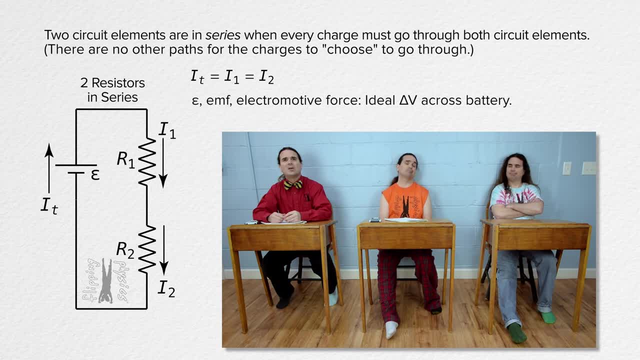 ideal electric potential difference across the battery. Right, It's an ideal battery with no internal resistance. Thanks, What does the t-subscript on the current mean? Oh, that means terminal, as in the current, through the terminals of the battery. Okay, Thanks. 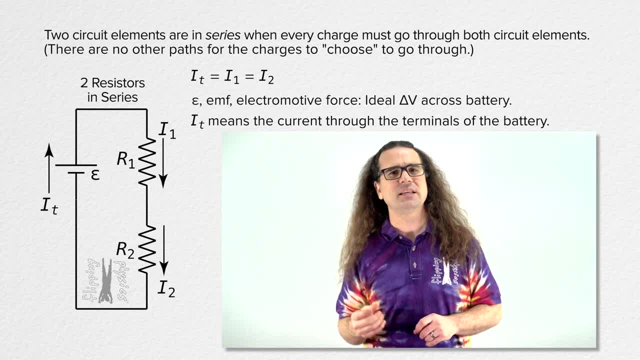 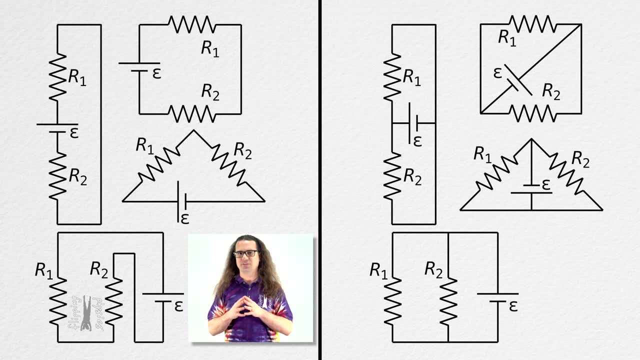 You're welcome. Thank you everybody. You know what actually, because identifying when circuit elements are in series can be confusing for students. let's take a moment to put eight example circuits on the screen. Each circuit has two resistors and one battery. All four circuits on the left side. 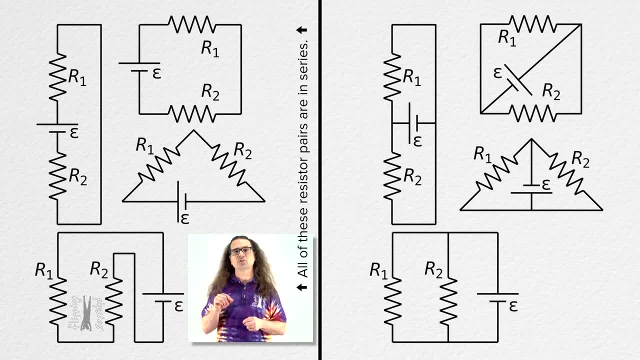 of the screen have two resistors in series. All four circuits on the right side of the screen have two resistors which are not in series. I'm not going to take the time to walk through each one of these examples right now, so if you want to pause the video for a moment to look over them, 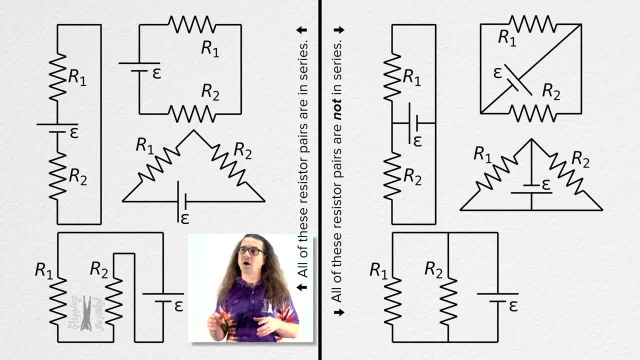 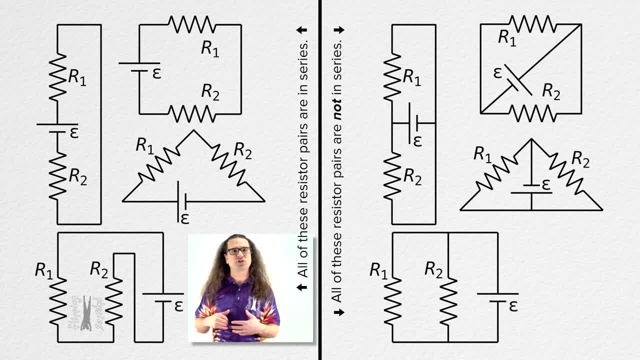 If you need more help understanding this, I do have a video which shows color-coded animations of circuits, which I think helps with understanding quite a bit. Now back to the circuit we were just working with. Actually, you know what I do want to mention that adding a third resistor. 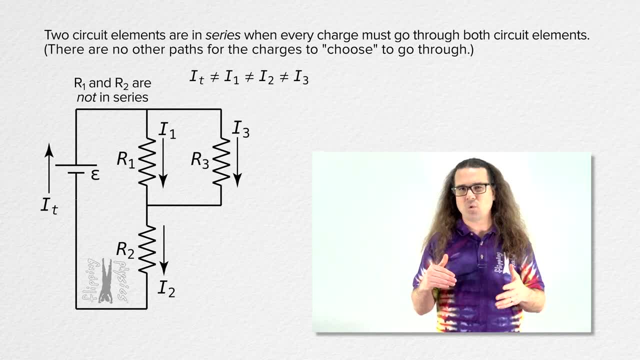 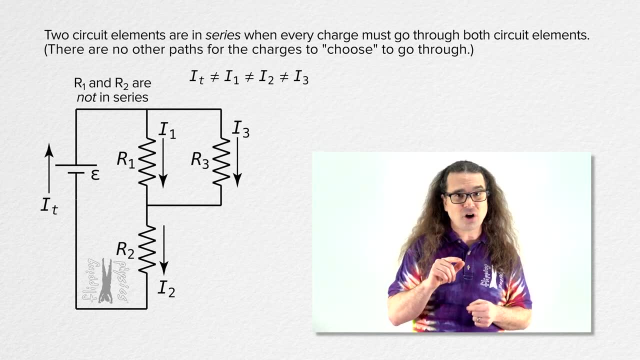 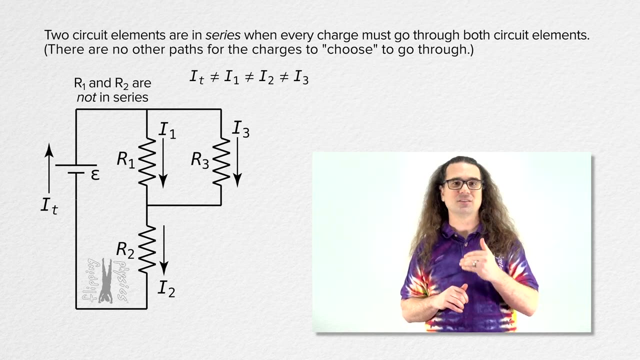 into this circuit like. this makes it so resistor 1 and resistor 2 are no longer in series. Between resistor 1 and resistor 2, an anthropomorphic charge would have a choice about which path to follow. So that makes it so: resistor 1 and resistor 2 are no longer in series. 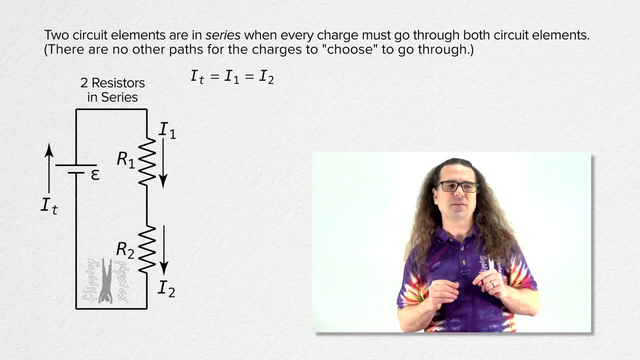 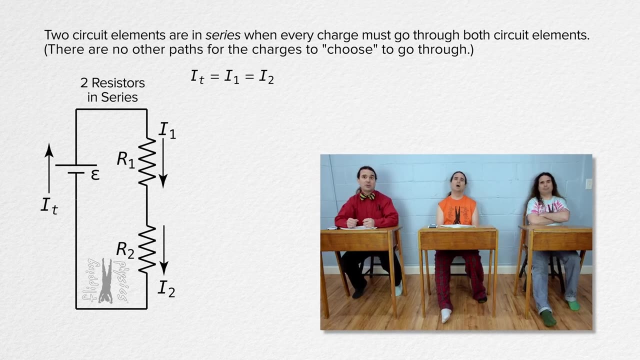 Alright, now I really mean it. Back to the circuit we were working with. Billy. tell what we know about the electric potential differences across all the circuit elements. in this circuit with two resistors in series with a battery, Certainly, And because these are ideal wires with zero resistance, the electric potential 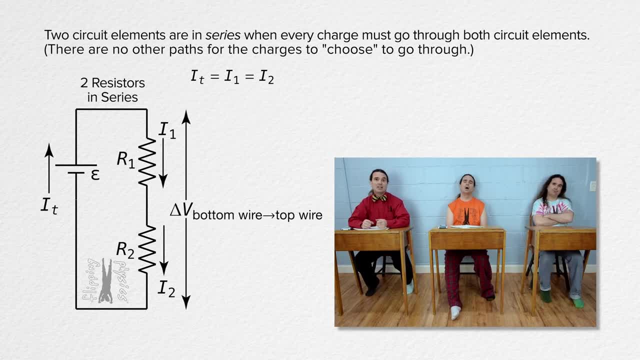 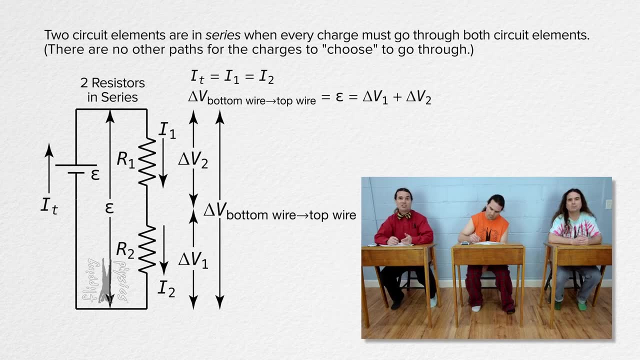 difference from the bottom wire to the top wire is the same as the electric potential difference across the battery, and it is the same as the electric potential difference across both resistors, which equals the summation of the electric potential differences across the two resistors. Thank you, Billy. 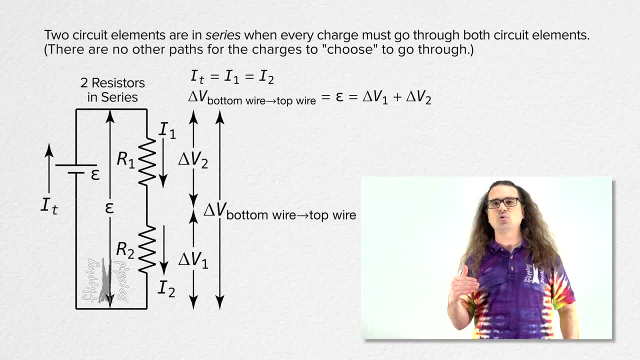 Realize we can get to the same equation by recognizing that if you go all the way around a loop in an electric circuit, the electric potential difference equals zero. For example, starting at point A, which is in the lower left-hand corner of the circuit, and going clockwise through the circuit all the way back to point A. 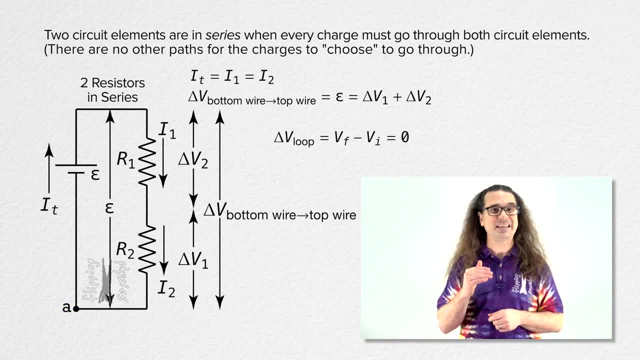 electric potential difference equals final electric potential minus initial electric potential. and if we start and end at point A, both of those are at the same electric potential and at the electric potential at point A, and the differences of those two equals zero because they're the same. 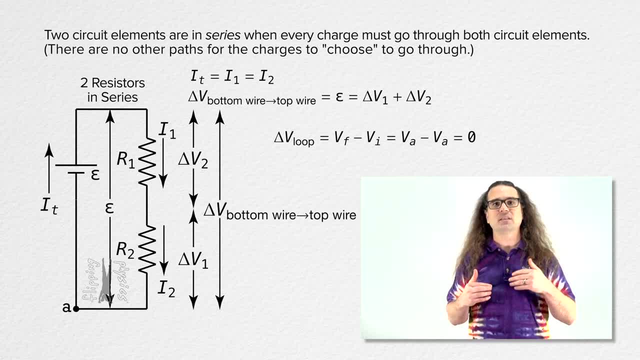 Going up from point A through the circuit, we have the electric potential difference across the battery, where equals the EMF of the battery and we're going in the direction of the current. therefore, we know that EMF, or electric potential difference, goes up when we go in the direction of the current across a battery. 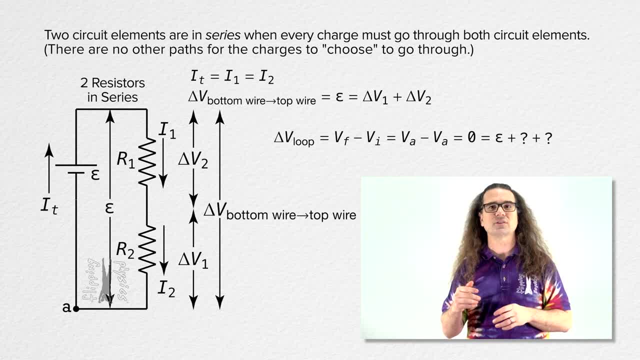 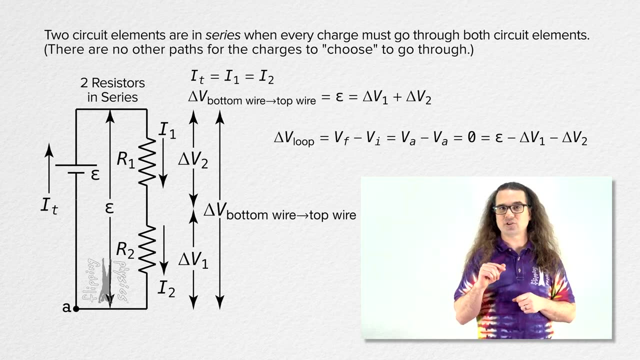 Next we have the electric potential difference across the two resistors. However, we showed last time that when going in the direction of current in a resistor, the electric potential goes down. So we subtract both electric potential differences across the resistors, Moving both of the electric potential differences across. 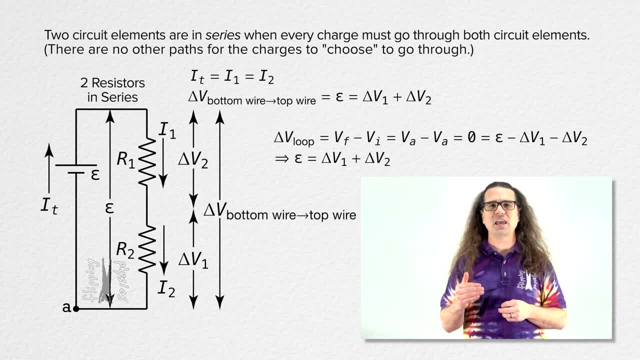 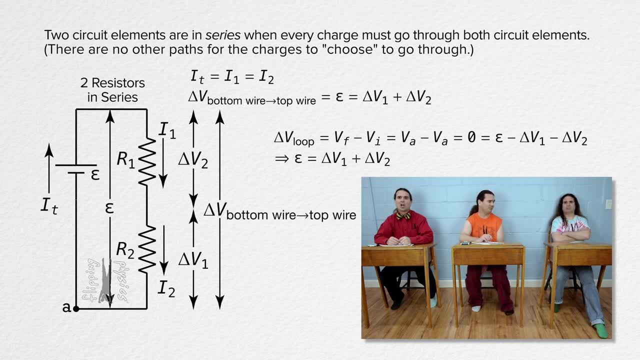 the resistors to the other side of the equation gives us the same equation Billy solved for. I like Billy's solution better. Billy's solution only took 57 words to explain. Yours took 236.. 57 words is a lot fewer than 236. 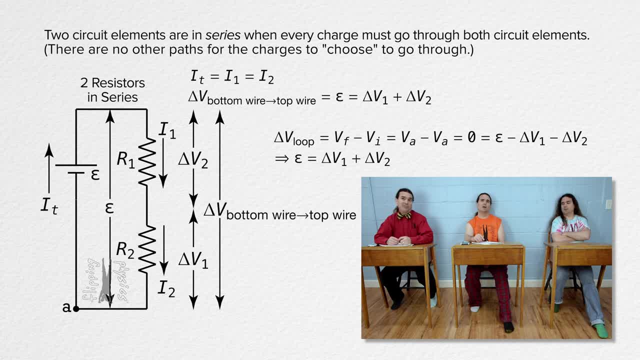 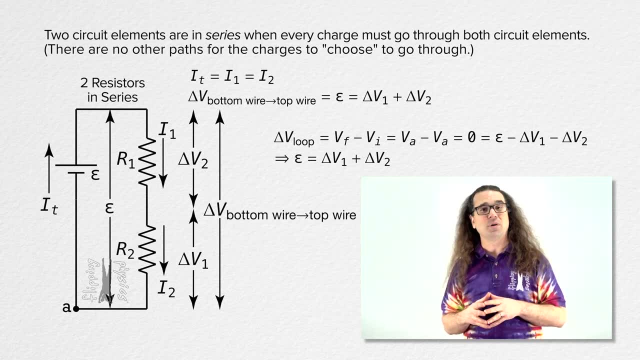 I'll take 57.. I like Mr P's solution too. Yeah, Either way, they are both correct, so it does not matter to me. Bobby, use Ohm's law with this equation And let's see what happens. 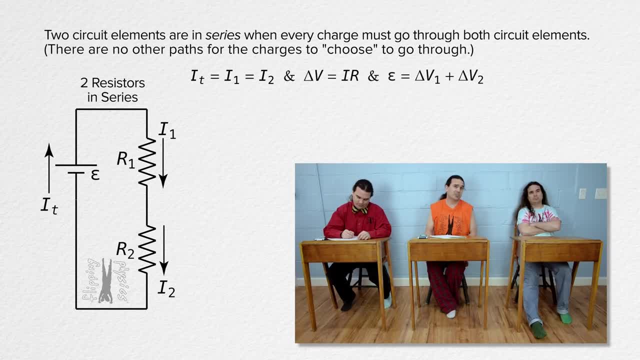 Okay, Ohm's law states that electric potential difference equals current times resistance. So we can substitute current times resistance in for each of the electric potential differences. in that equation The subscripts for the two resistors are 1 and 2 for the current through and the resistance of each resistor. 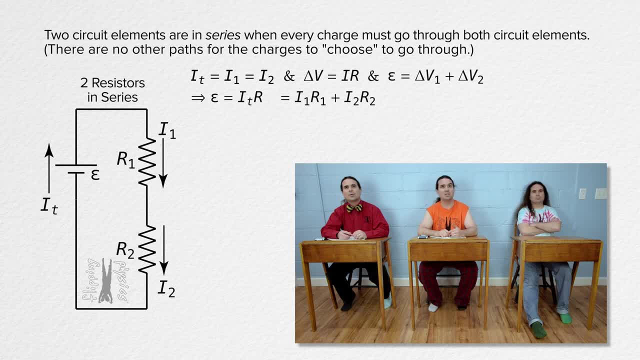 For the current through the battery, let's use a subscript of t, like you did before for the current through the terminals of the battery. For the resistance of the battery: you said it is an ideal battery, so it has zero resistance, right? 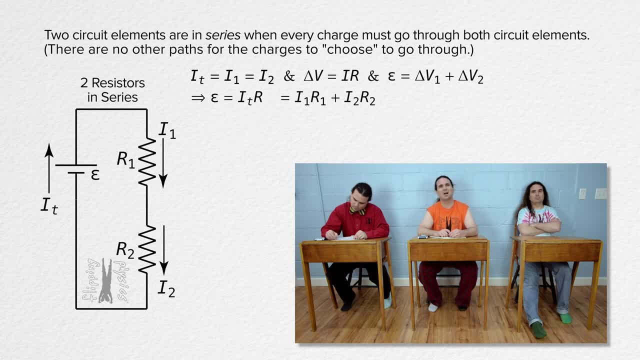 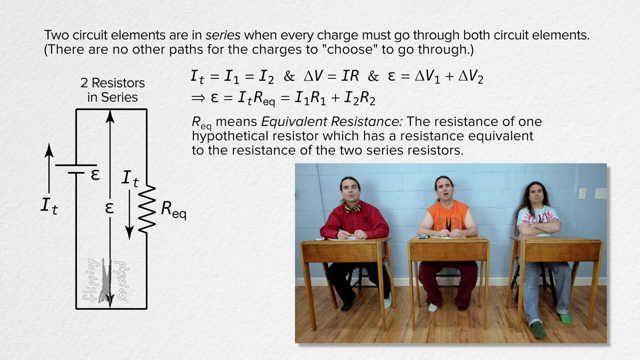 But that doesn't really make sense. Let's use a subscript of eq for the resistance there. That eq subscript means equivalent, In other words the current through the battery times, the resistance of one hypothetical resistor which has a resistance equivalent to the resistance of the two series resistors. 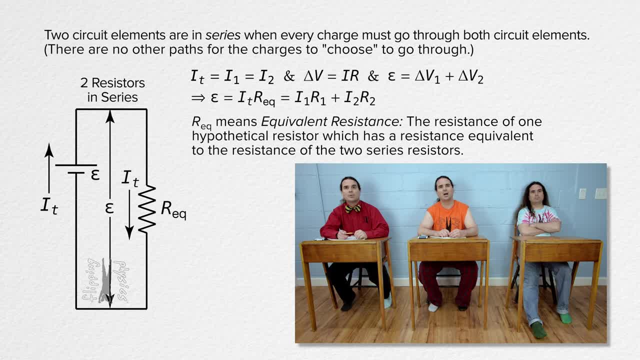 equals the emf across the battery. Again, this is just Ohm's law: Electric potential difference equals current times resistance. It's just that the electric potential difference across the battery, the emf, has the same magnitude as the electric potential difference across a resistor equivalent to the two series resistors. 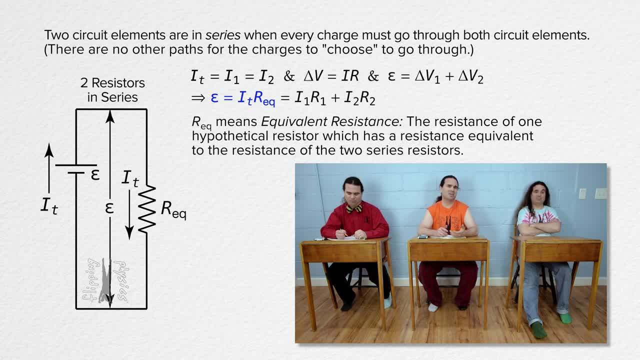 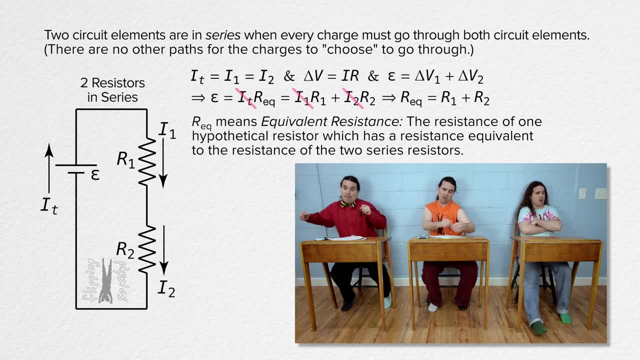 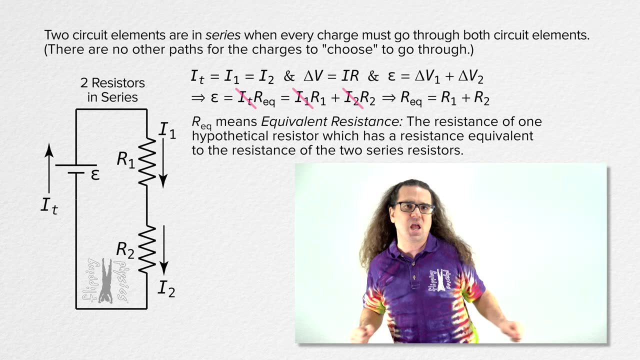 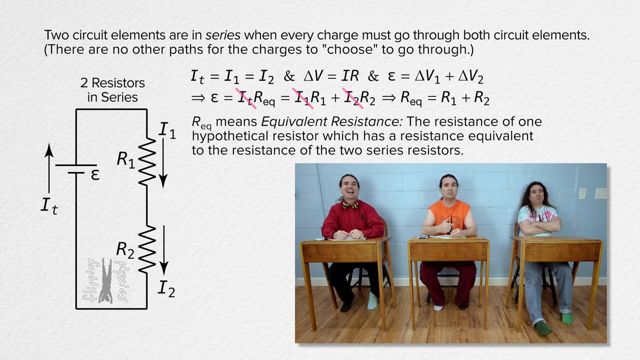 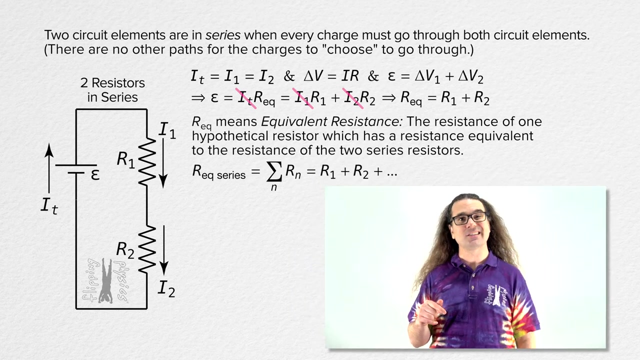 That makes sense. But um, All the currents are equal. so Everybody brought current to the party, Everybody brought mass. That means a resistor with the resistance equivalent to the two series resistors equals resistance 1 plus resistance 2. Right, And a more general equation for the equivalent resistance of n, a variable number of resistors in series. 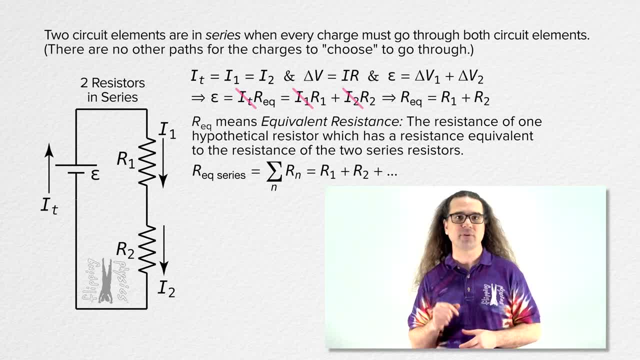 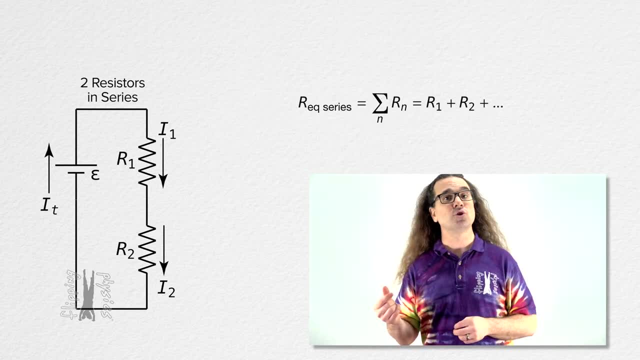 equals the summation of the resistances of n number of resistors. You just add up the resistances of all the series resistors. All right, Let's move on to two resistors in parallel. Again, let's use an anthropomorphic charge. 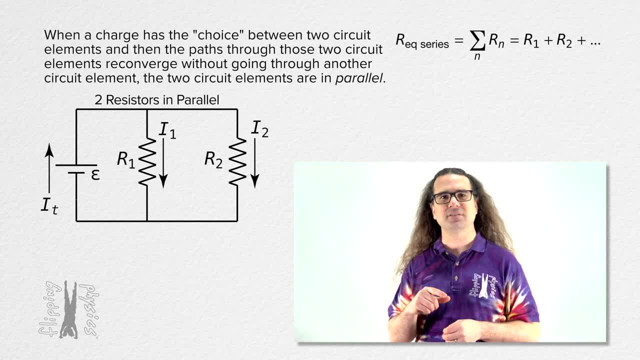 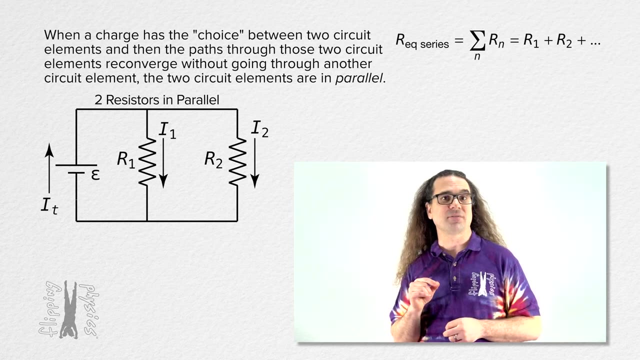 An anthropomorphic charge has the choice between paths that go through the two resistors, And then those two paths join back again without going through any other circuit elements. That is why these two resistors are in parallel. Notice, then, that the electric potential differences across all three of these circuit elements are equal. 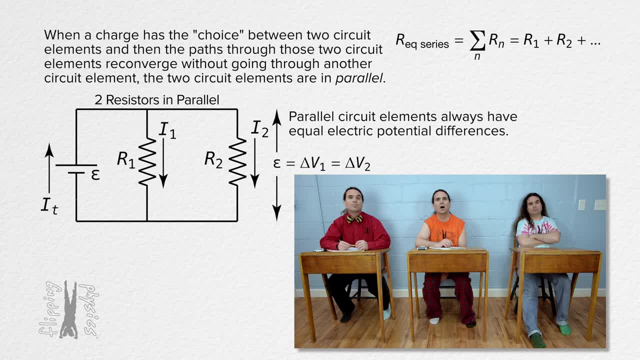 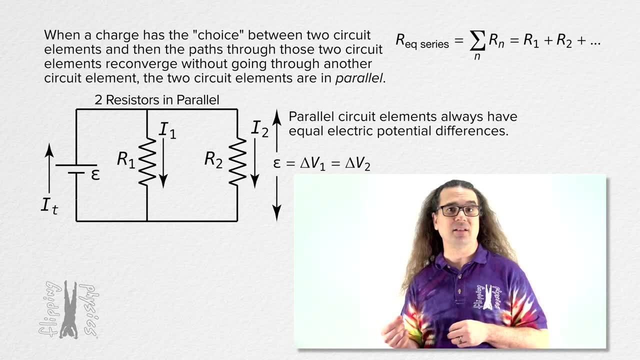 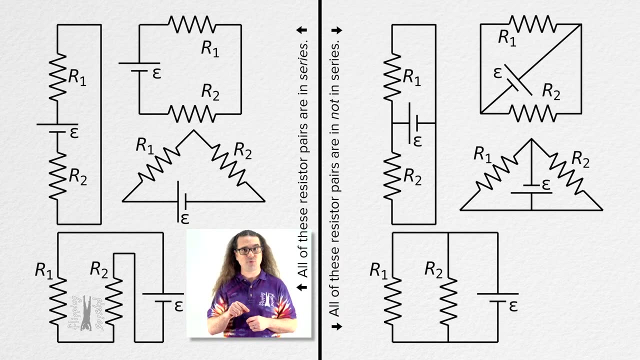 This is always true, but it's not always true. It's not always true of circuit elements which are in parallel. They always have equivalent electric potential differences. Now, because identifying when circuit elements are in parallel can be confusing for students, let's take a moment to put the same eight example circuits on the screen that I did before. 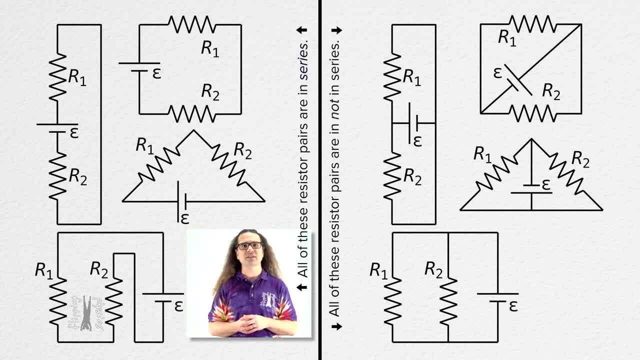 All four circuits on the left side have two resistors in series and all four circuits on the right side have two resistors which are in parallel. Again, I'm not going to take the time to walk through each one of these examples, so if you want to pause the video for a moment to look over them for yourself, 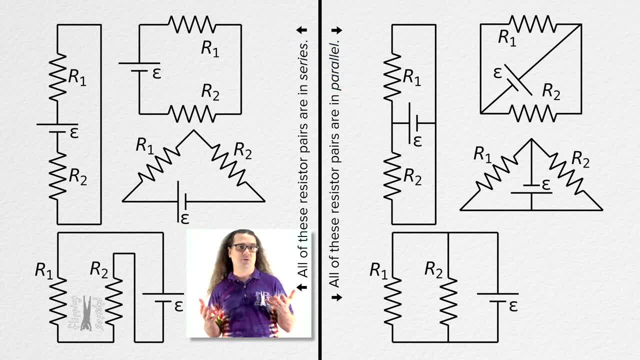 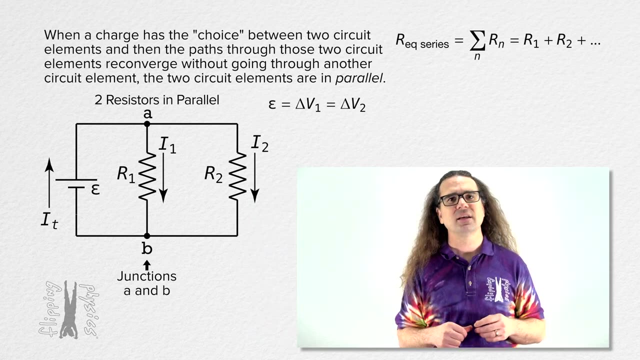 feel free to do so Again. if you need more help understanding this, I do have another video which shows color-coded animations of more circuits, which I think helps with understanding these circuits. Now back to the circuit we were working with Billy. use what we know about the two junctions in this circuit. 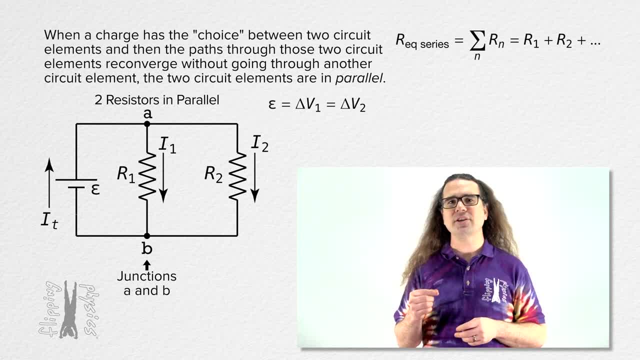 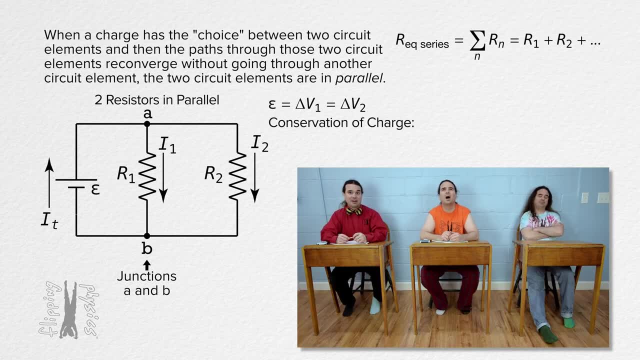 which I have labeled a and b, to derive the equation for the equivalent resistance of two resistors in parallel. Please, Absolutely, Because conservation of charge states that every charge which goes into a junction will also come out of that junction. the current into a junction equals the current coming out of a junction. 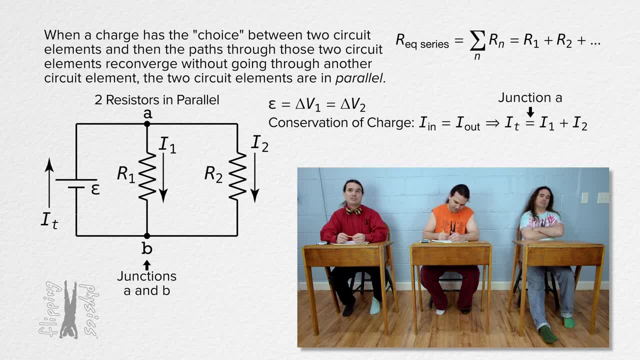 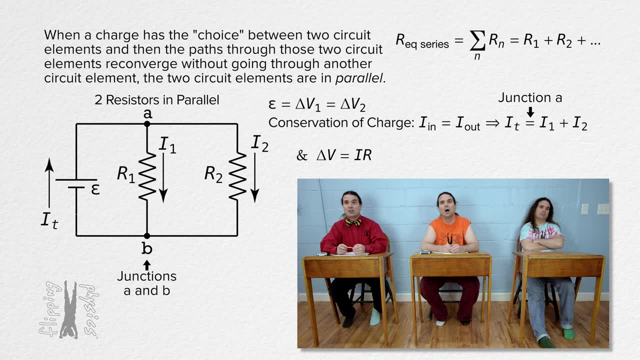 Therefore, for junction a the current through the terminals of the battery equals the sum of the two currents going through the two resistors. From Ohm's law we know current equals electric potential differences divided by resistance and we can substitute that in for each current in our previous equation. 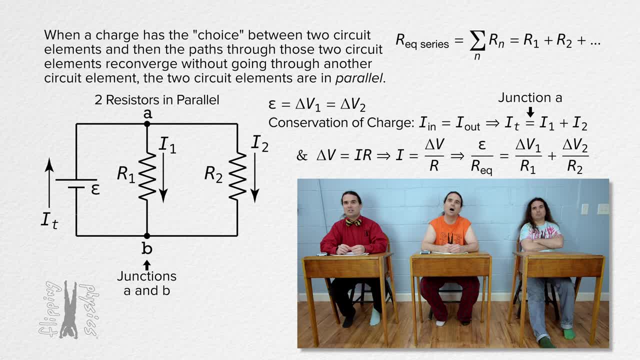 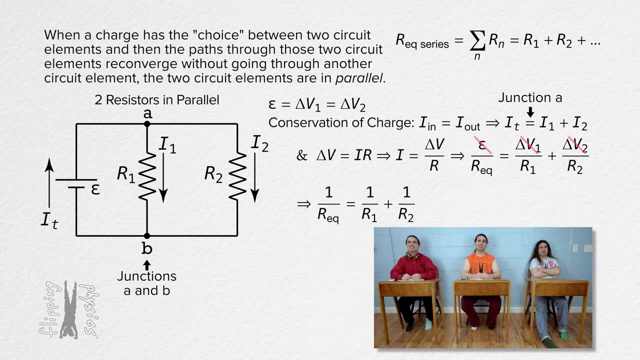 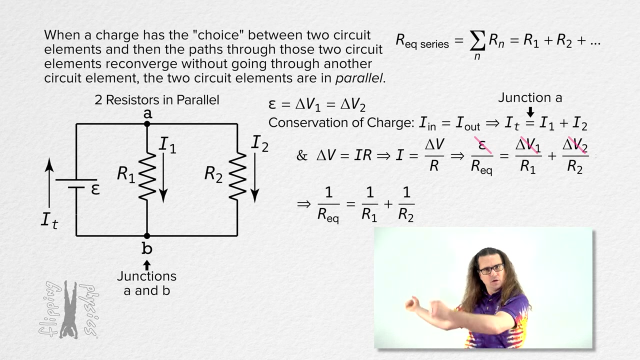 That means emf over equivalent resistance equals the sum of the electric potential differences across each resistor divided by the resistance of each resistor. All the electric potential differences are equal. so everybody brought electric potential difference to the party. all the electric potential differences are equal, so everybody brought electric potential difference to the party. 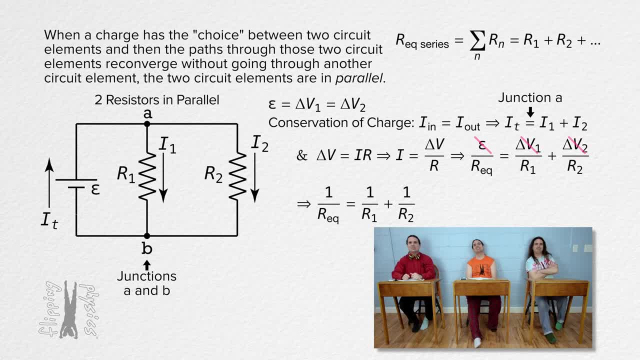 Everyone brought electric potential differences to the party into equal sum of the go levelかった. That means one resistor with the equivalent resistance of two resistors in parallel equals the inverse of the sum of the inverses of the resistances of the two parallel resistors. 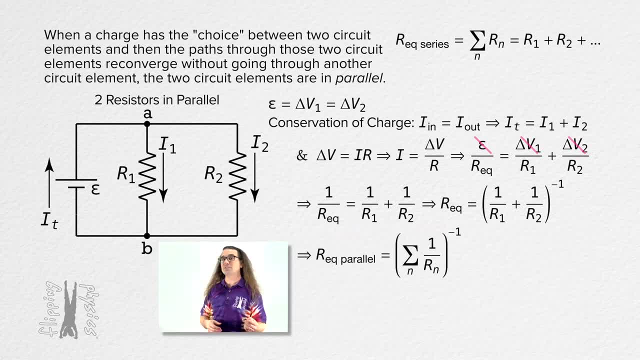 Exactly And a more general equation: for the equivalent resistance of n a variable number of resistors in parallel equals the inverse of the sum of the inverses of the resistances of n numbers of resistors. You just add up the inverses of the resistances of all the parallel resistors and take the inverse of that. 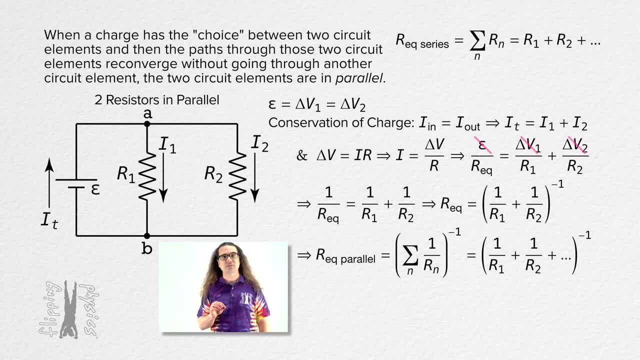 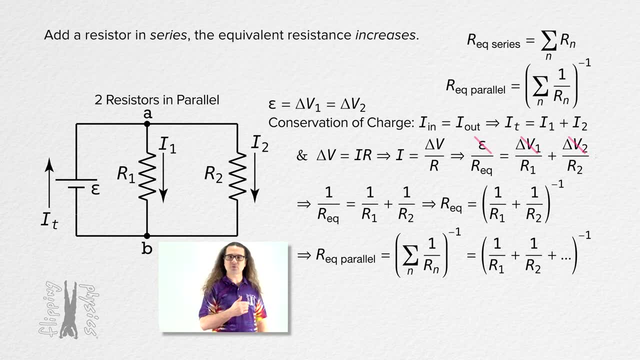 Now looking at the general concept of resistors in series and in parallel. from the equations you can see that when we add resistors in series, the equivalent resistance goes up, And when we add resistors in parallel, the equivalent resistance goes down. 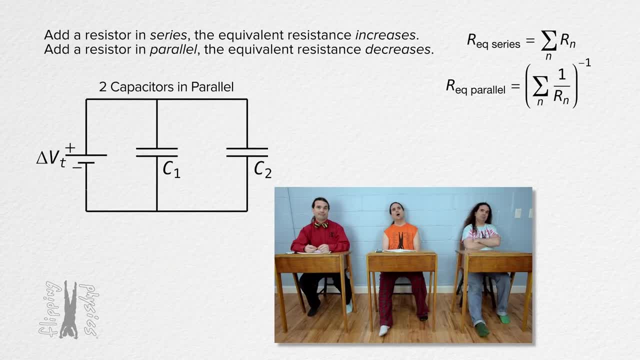 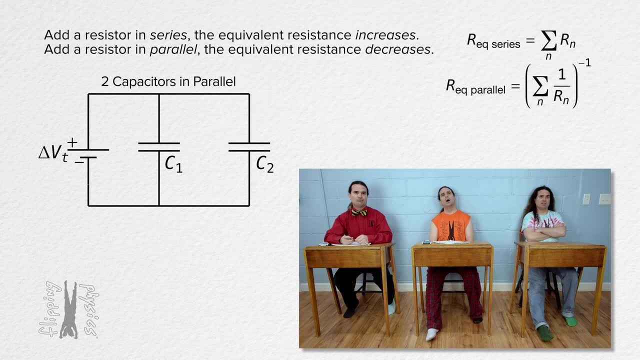 Now let's look at two capacitors in parallel. Bo see what you can do with two capacitors in parallel. Well, those two capacitors are in parallel. Then we know all the electric potential differences are equal in magnitude. Hold up. 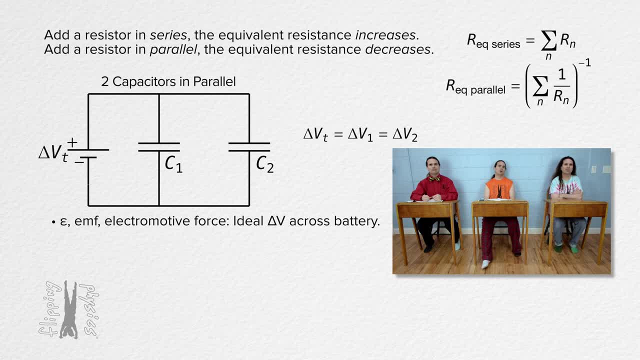 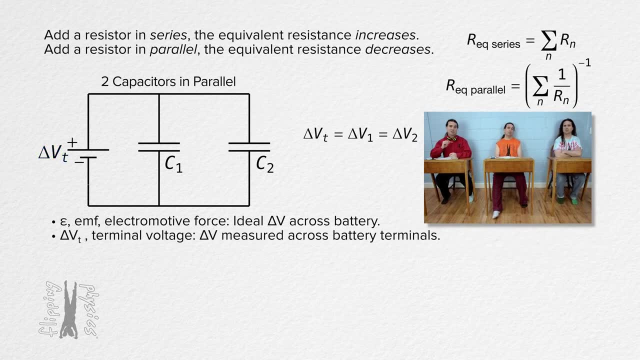 What happened to the EMF of the battery? Now we have an electric potential difference with a T subscript instead. What is that? That is the terminal voltage, Which is the electric potential difference measured across the terminals of the battery And whenever the battery is supplying current to a circuit. 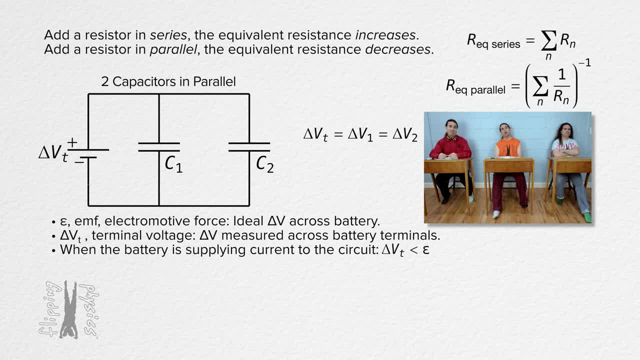 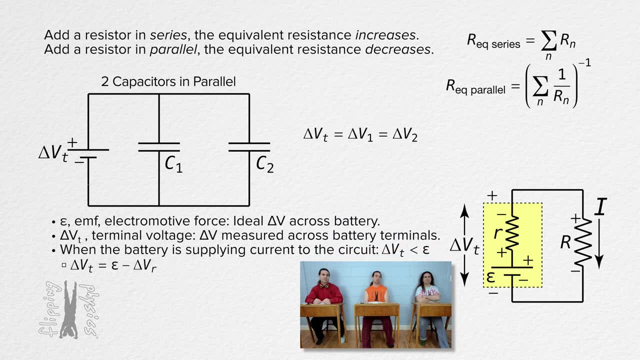 the terminal voltage is less than the electromotive force, or EMF, of the battery, Because all real batteries have internal resistance which decreases the voltage measured across the terminals of the battery. Yep Terminal voltage equals EMF minus current through the battery times. the internal resistance of the battery: lowercase r. 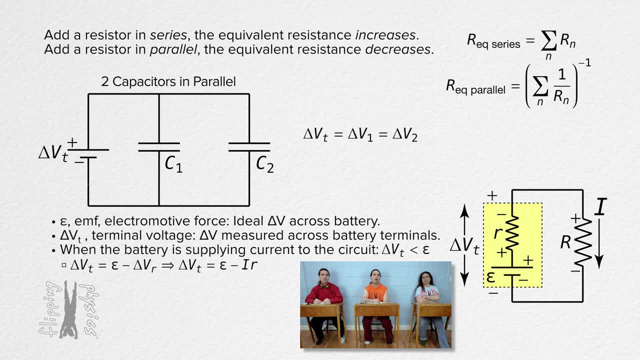 Which means, as the current through the battery increases, the terminal voltage across the battery decreases. Okay, sure, I remember that now, But why would he switch it from EMF to terminal voltage in the middle of a lecture like this, So we can review? 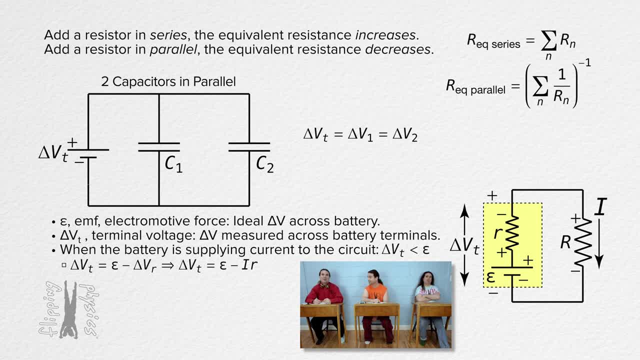 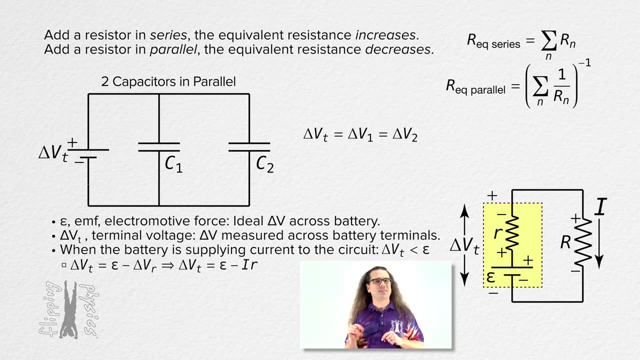 Mr P never misses an opportunity to do a quick review. No, That does not sound like me Right. Definitely not, Nope. Anyway, Two capacitors in parallel with a battery, All the electric potential differences are the same. Think about the charges moved by the battery to the plates of the capacitors. 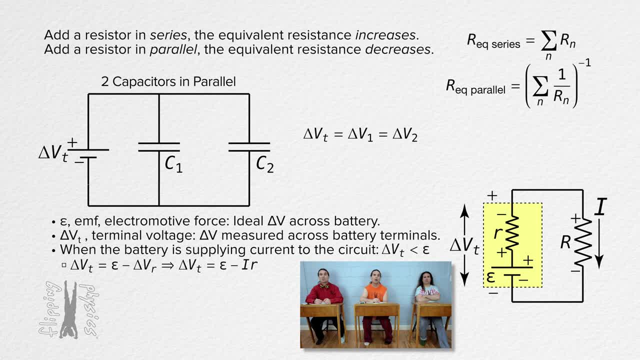 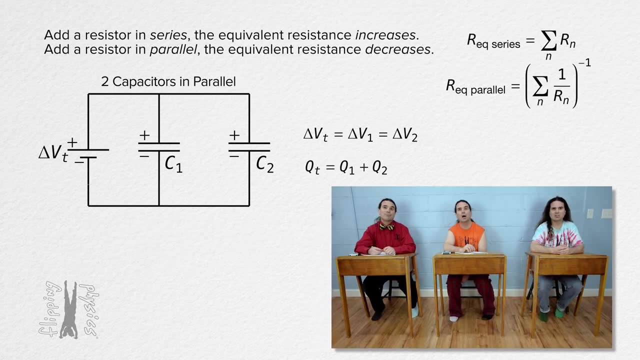 Sure, Because the charges moved by the battery to the top plates of the capacitor need to go to either capacitor 1 or capacitor 2, the charge moved by the battery to the plates of the capacitors equals the sum of the charges on the capacitors. 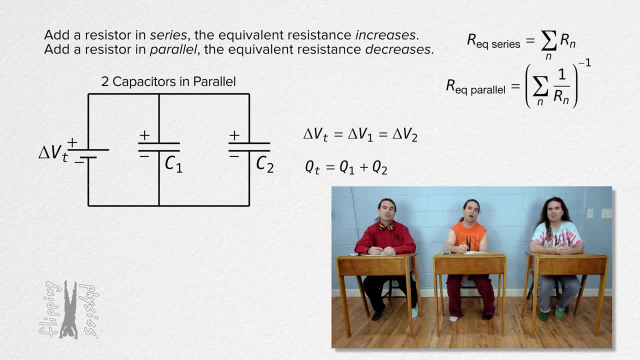 And now we can use the definition of capacitance. Capacitance equals the magnitude of the charge stored on one of the plates of the capacitor over the electric potential difference across the plates of the capacitor. Yes, That means charge equals capacitance times electric potential difference. 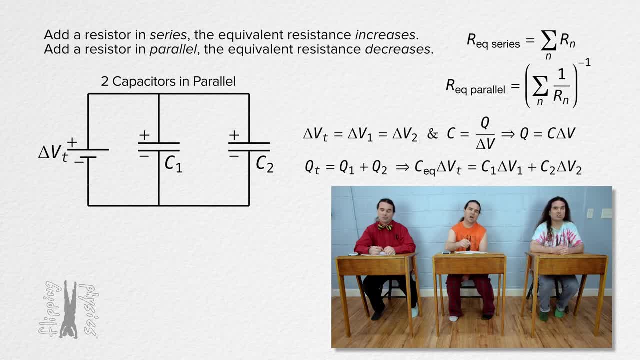 Which we can substitute into the charge equation to get equivalent capacitance times. terminal voltage equals the sum of the capacitance of each capacitor times the electric potential difference across each capacitor. And Because the electric potential differences are all equal, Everybody brought electric potential difference to the party. 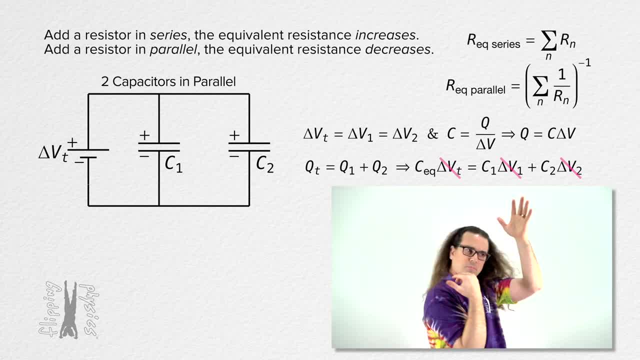 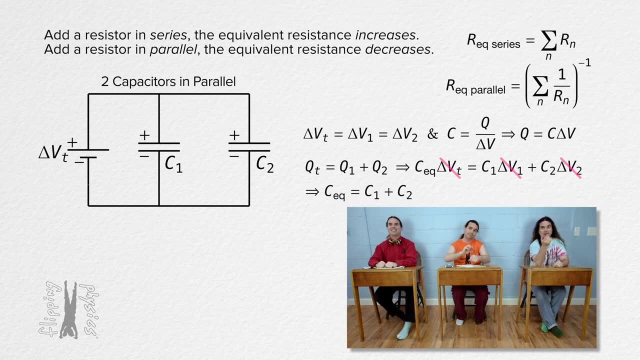 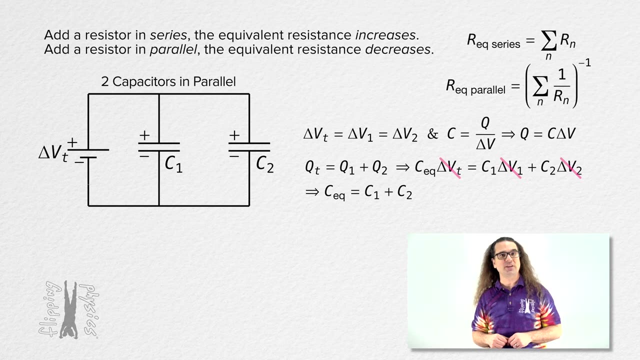 And we get that the equivalent capacitance of two capacitors in parallel equals the sum of the capacitance of the two parallel capacitors. Correct Bo And a more general equation: for the equivalent capacitance of n a variable number of capacitors in parallel equals the summation of the capacitance of n number of capacitors. 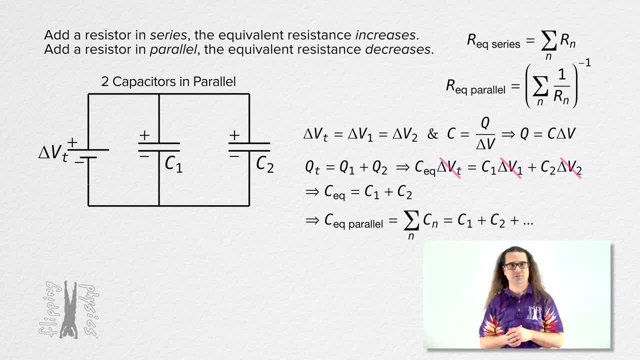 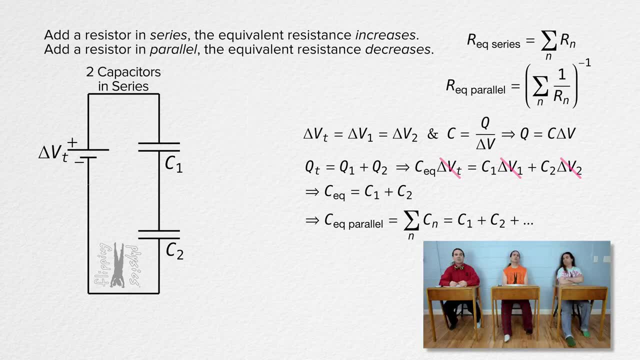 You just add up the capacitance of all the parallel capacitors. Alright, let's move on to two capacitors in series. Bobby, it's your turn again. Okay, We know. the electric potential difference equation is the same as for two resistors. 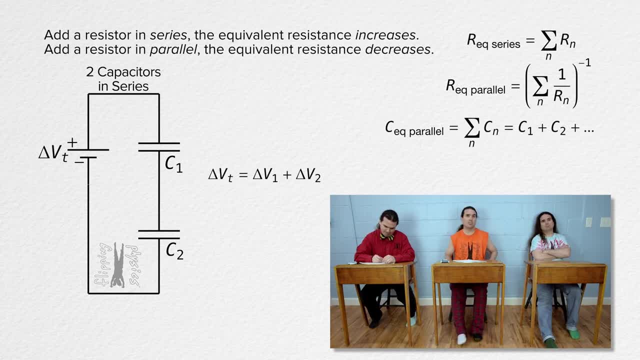 in series. Terminal voltage equals voltage across capacitor 1 plus voltage across capacitor 2.. And looking at the charges moved by the battery to the plates of the capacitors, well we know the magnitude of the charge moved by the battery to the top plate of capacitor. 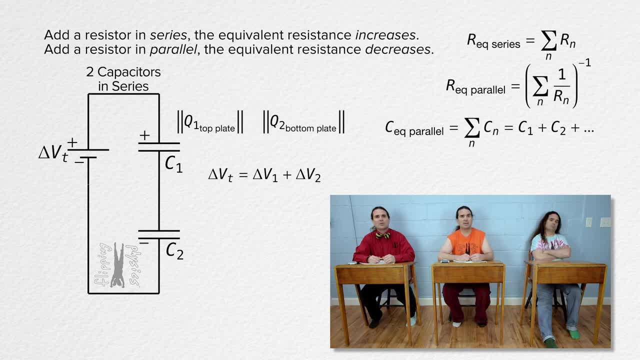 1 and the magnitude of the charge moved to the bottom plate of capacitor 2 are equal in magnitude. But what happens then? I mean, how would any charge get on the bottom plate of capacitor 1 and the top plate of capacitor 2?? 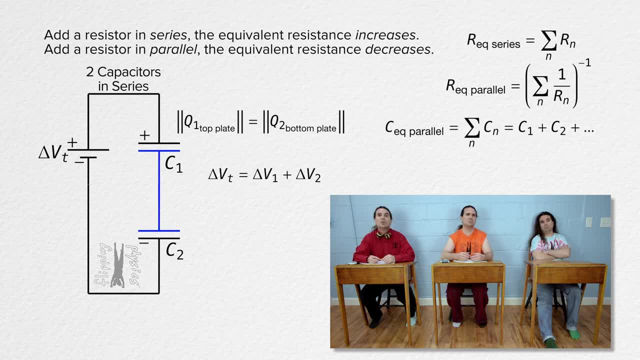 Those two plates are connected by a wire and that whole system is not physically connected to any part of the circuit. There are already electrons. The electric charge is located there, on the wire and the two plates of the capacitor right. Okay, Yes. 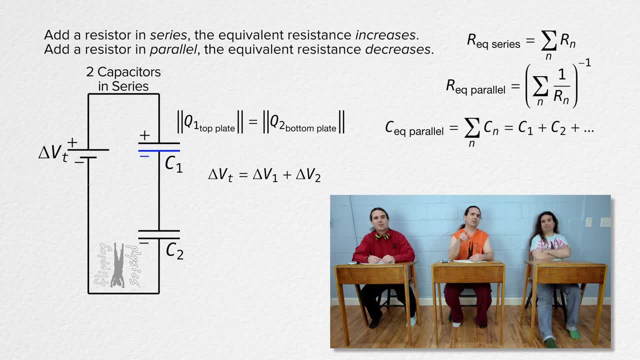 So negative charges are pulled to the bottom plate of capacitor 1 by the positive charges on the top plate of capacitor 1.. And positive charges are pulled to the top plate of capacitor 2 by the negative charges on the bottom plate of capacitor 2.. 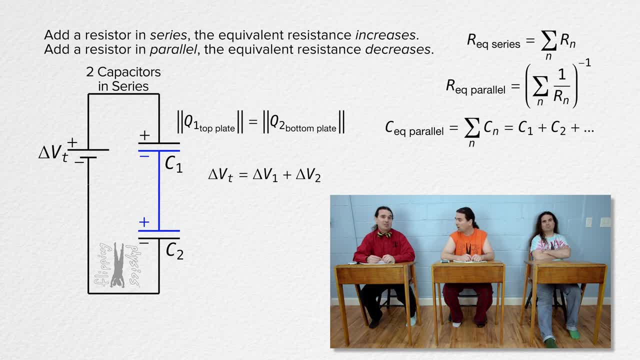 That's cool, Yeah. That area gets polarized by the top plate of capacitor 1 and the bottom plate of capacitor 2.. That is cool, Yeah, And that means that the charges on all the plates of those capacitors are equal in magnitude. 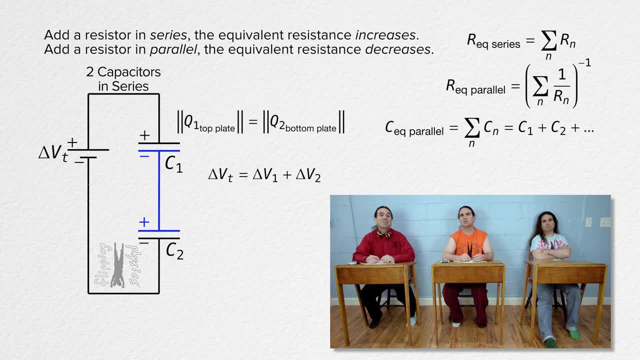 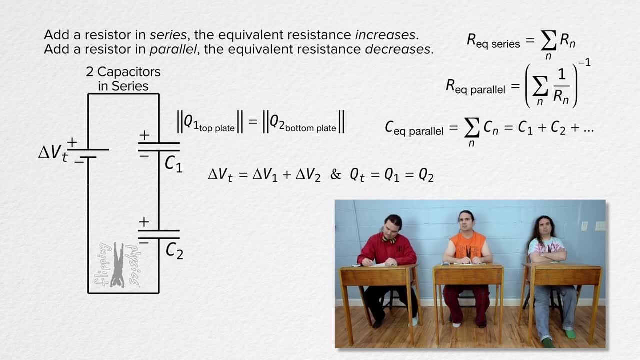 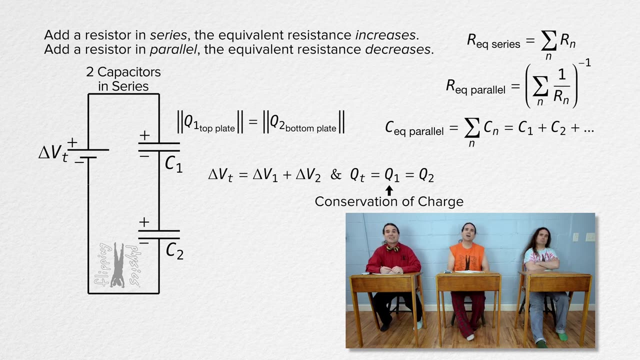 In other words, the total charge moved by the battery equals the charge on capacitor 1, which equals the charge on capacitor 2.. That's basically just conservation of charge, Right, Mr P? Exactly, Bobby, Yeah, Okay, Uh. 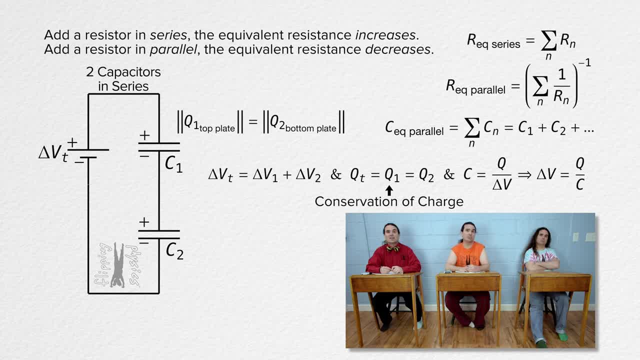 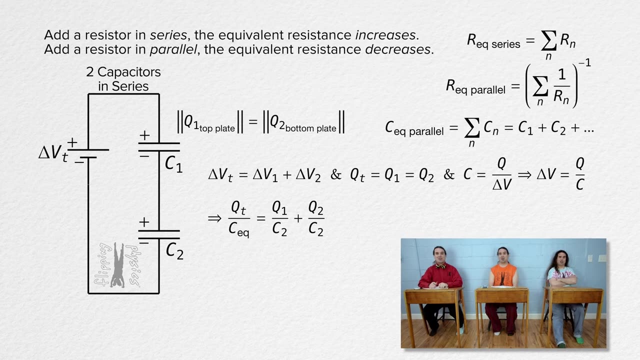 So we can show: the electric potential difference across a capacitor equals the magnitude of the charge on one of the plates of a capacitor over the capacitance of the capacitor. We can substitute that into our electric potential difference equation. All the charges are the same. so everybody brought charge to the party. 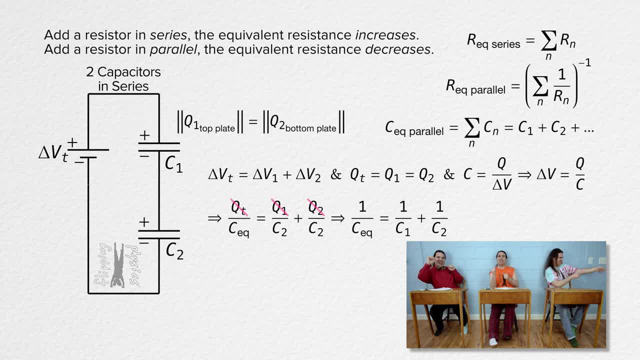 We are partying a lot today. Yes, we are. I like it. Everybody brought mass. Mass, That means one capacitor with an equivalent capacitance of two capacitors in series equals the inverse of the sum of the inverses of the capacitance of the two series capacitors. 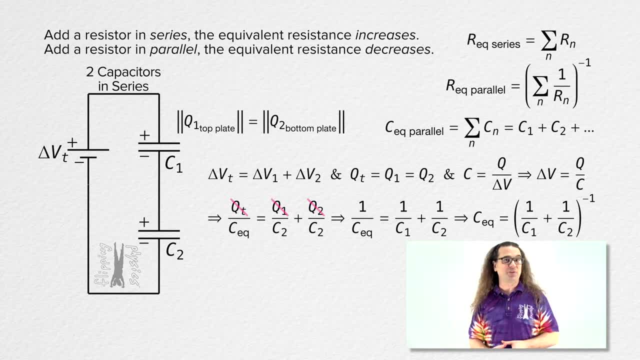 Perfect, Bobby, Thanks. And a more general equation: for the equivalent capacitance of n, a variable number of capacitors in series equals the inverse of the sum of the inverses of the capacitance of n number of capacitors. You just add up the inverses of the capacitances of all the series capacitors and you get the 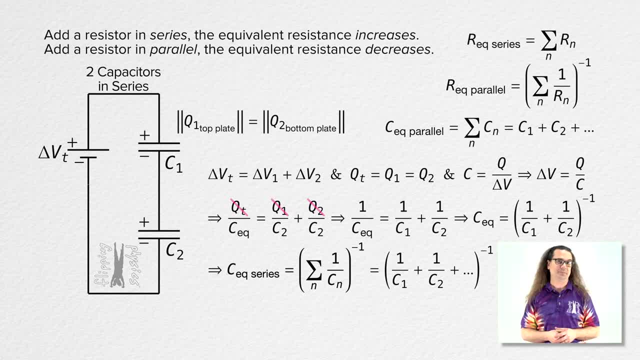 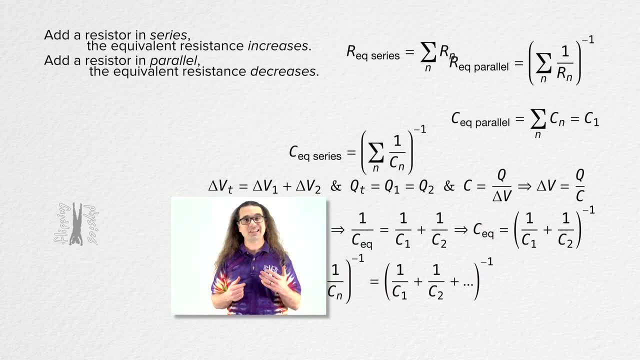 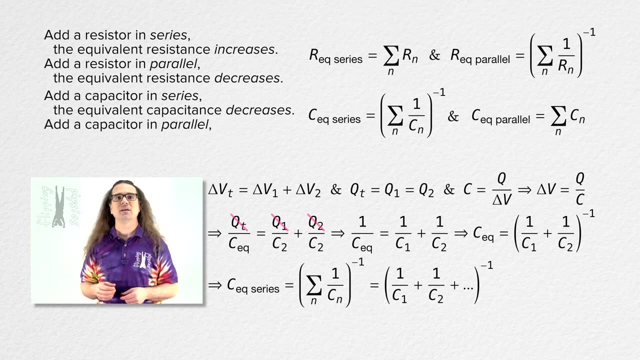 result. Now, looking at the general concept of capacitors in series and in parallel, from the equations you can see that when we add capacitors in series, the equivalent capacitance goes down, and when we add capacitors in parallel, the equivalent capacitance goes up. 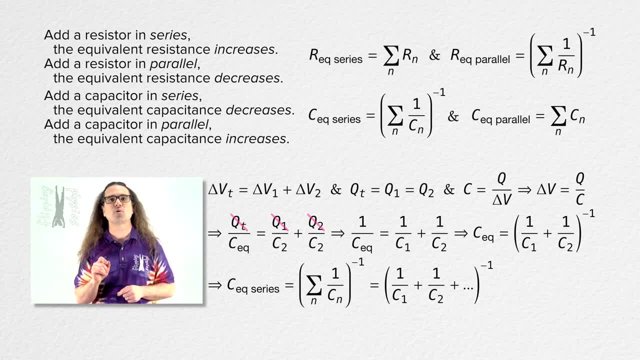 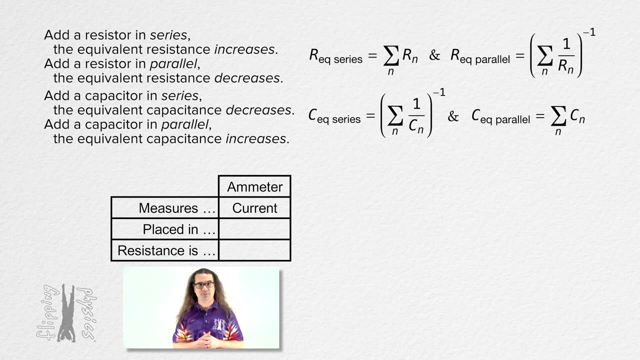 Please notice: the series and parallel equations for resistors and capacitors are reversed. Now let's discuss how to use the tools which measure current at electric potential difference, starting with the ammeter, which measures current or number of amps. We need to decide if an ammeter needs to be put in series or parallel with the circuit. 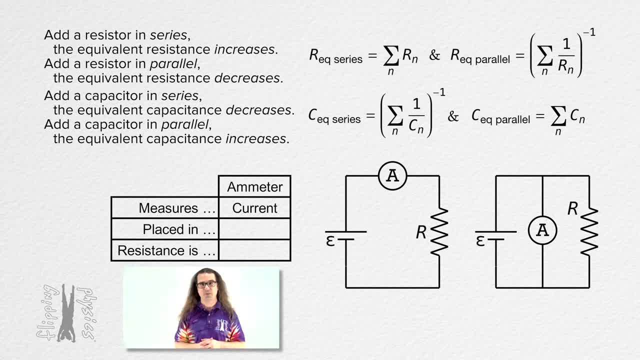 element it is meant to measure the current through. So let's look at what happens when we attempt to measure the current through a resistor using an ammeter in series and in parallel with a resistor. Billy, tell me what you see, Yep. 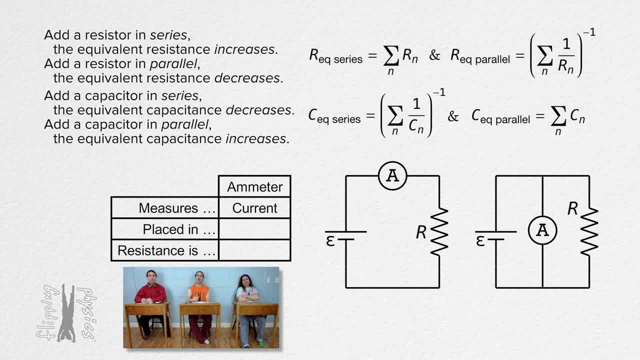 I can do that. Well, it looks like when you put an ammeter in parallel with a resistor, the charges which go through the ammeter will be different from the charges which go through the resistor. so putting an ammeter in parallel with a resistor will not actually measure the current through. 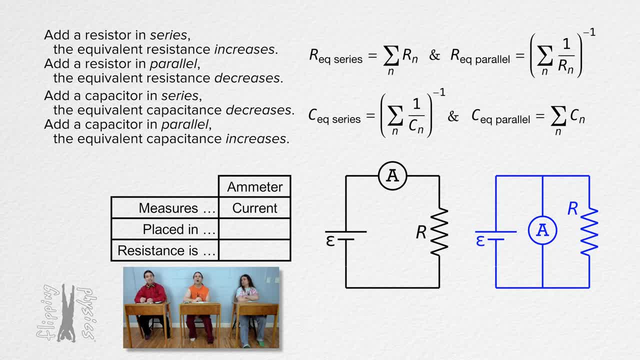 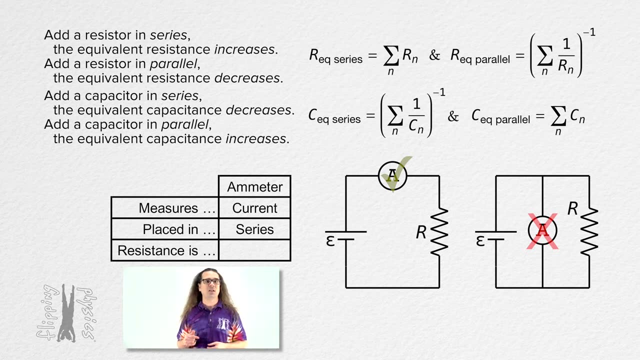 the resistor. so an ammeter needs to be placed in series with the circuit element. you are trying to measure the current through Correct Billy, And notice that the resistance of an ammeter needs to be very, very small. In this example circuit, if the resistance of the ammeter is not very, very small, the 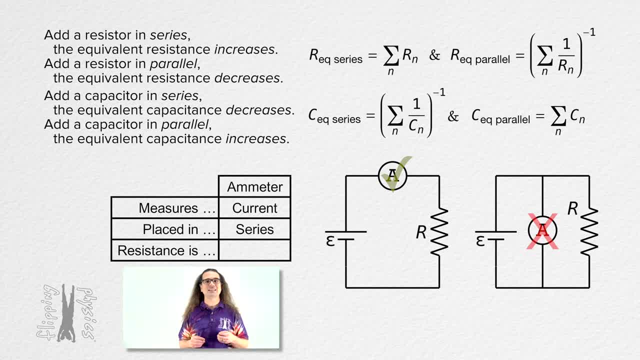 ammeter will increase the equivalent resistance of the circuit and decrease the current through the resistor you are trying to measure the current through. So, unless otherwise indicated, ammeters in this class are considered to have zero resistance. And I'll just mention that because ammeters have such a low resistance. if you accidentally 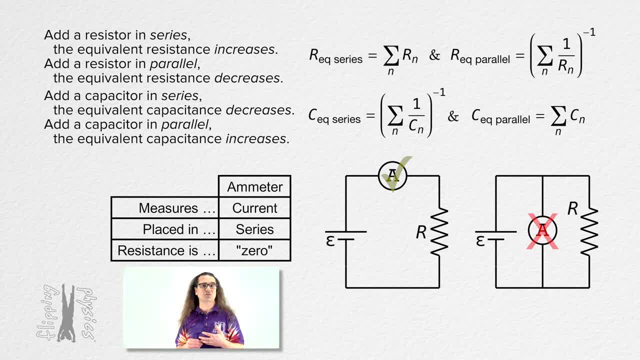 place an ammeter in parallel with the electric load of a circuit, the resistance will be very, very small. You are significantly decreasing the resistance in the electric circuit, which can significantly increase the current in the electric circuit and this can really damage equipment. 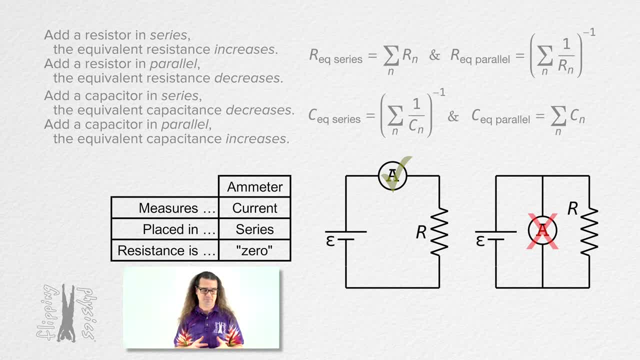 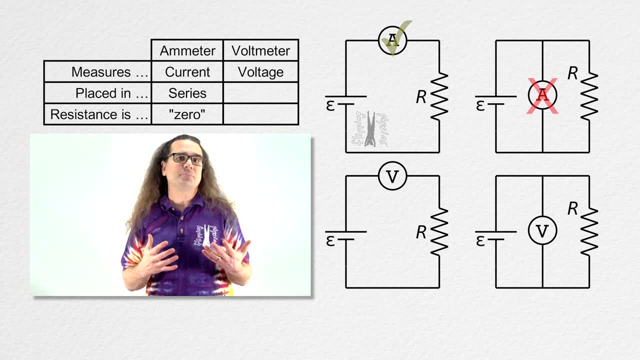 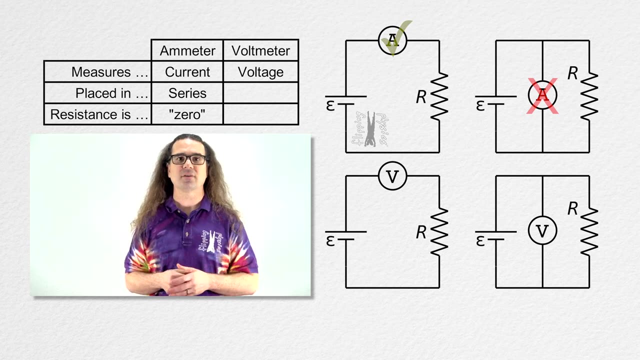 So please never put an ammeter in parallel. Now let's switch to a voltmeter which measures electric potential differences or voltage. Let's attempt to measure the electric potential difference across a resistor using a voltmeter, either in series or in parallel with a resistor. 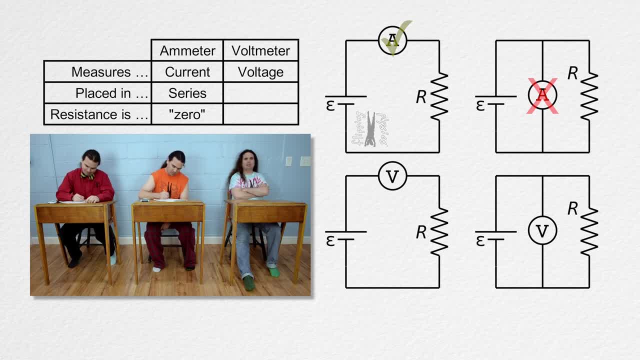 Bo, tell me what you see. Sure, Placing a voltmeter in series with a resistor actually does not measure the voltage across the resistor. I mean, the voltmeter and the resistor would have different electric potential differences. so I guess you have to place a voltmeter in parallel with the circuit element across which? 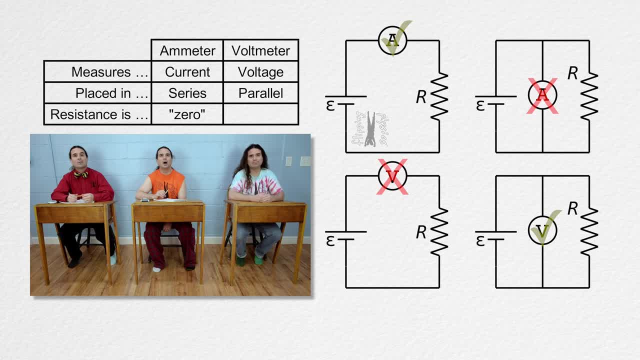 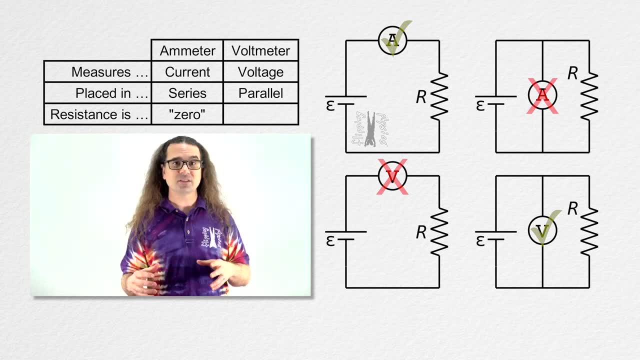 you are trying to measure the electric potential difference, Correct, Bo? Also notice that the resistance of a voltmeter needs to be very, very large. Okay, In this example circuit, if the resistance of the voltmeter is not very, very large? 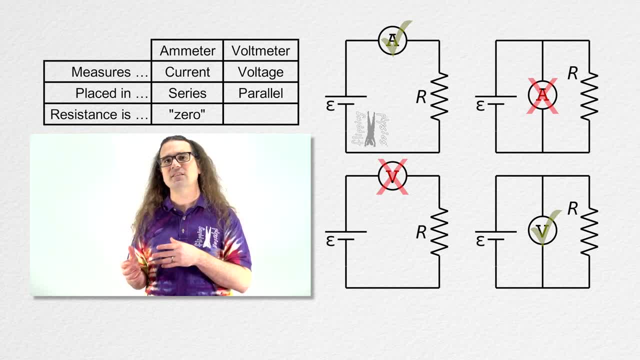 the voltmeter will provide a parallel path and decrease the equivalent resistance of the circuit, and that will increase the current delivered by the battery, which changes the way this electric circuit behaves. The tools you use to take measurements should not change the circuit you are attempting. 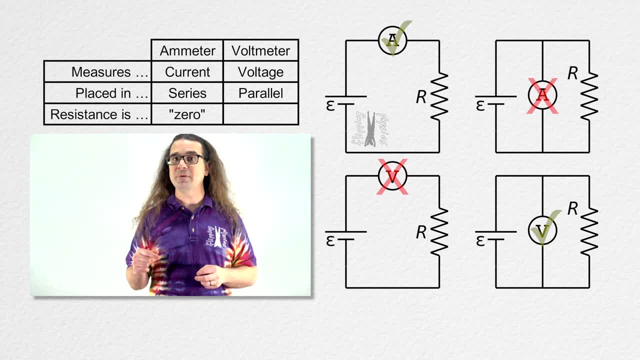 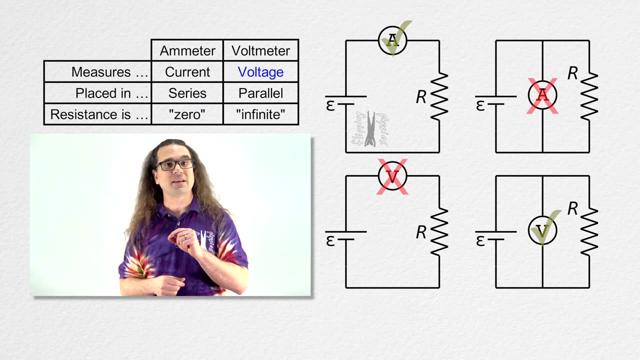 to measure. so, unless otherwise indicated, voltmeters in this class are considered to have infinite resistance. To review: m meters measure current are placed in series with the circuit element. you are measuring and have nearly zero resistance. Voltmeters measure electric potential difference are placed in parallel with the circuit element.